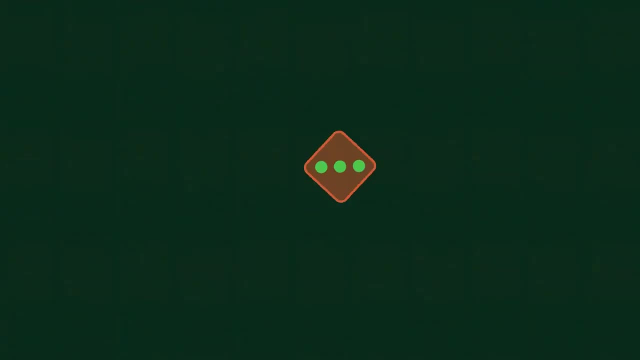 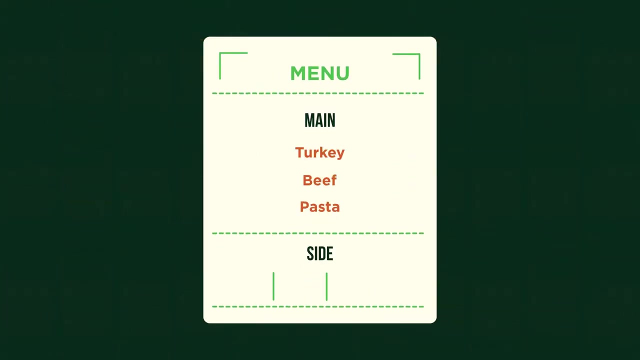 Consider a standard dice When rolled once. the sample space for this would be 1,, 2,, 3,, 4,, 5 and 6.. Any of these outcomes are possible. Now imagine yourself at a restaurant where you have the choice of turkey beef or pasta for main, with the option of chips, salad or vegetables on the side. 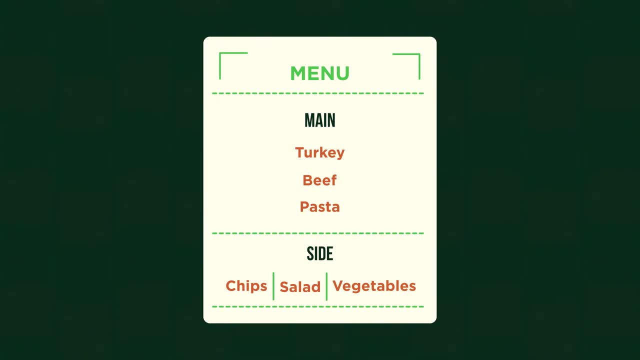 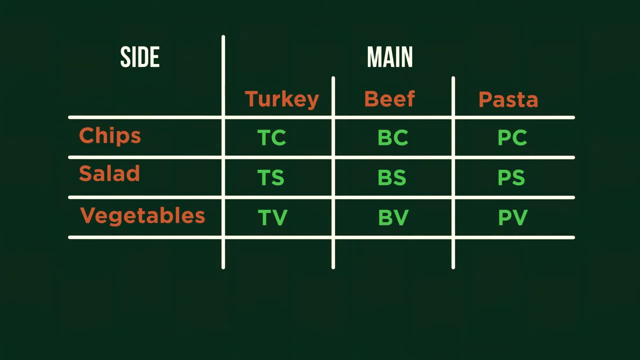 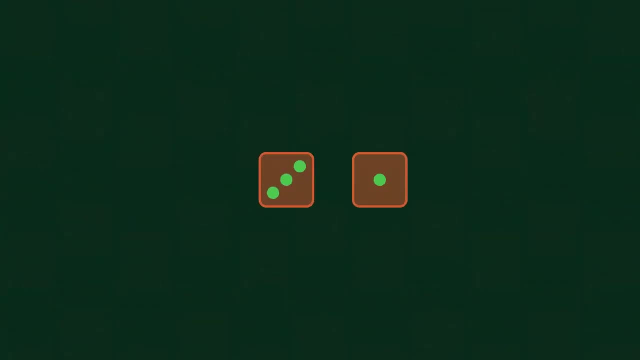 We can list the outcomes for this, as there are only nine, but we can also present them in a table like this. This form of sample space diagram is very useful, especially if you have to answer probability questions based on two events, For example with two dice. we could set up a table like this: 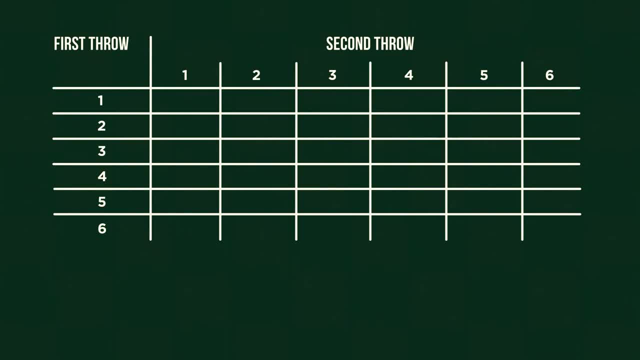 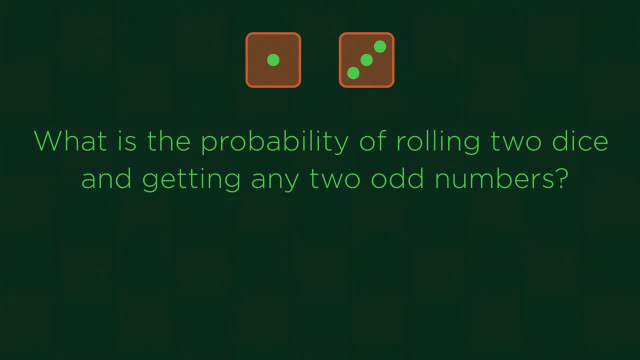 And then use it to answer multiple questions. Let's have a look at an example. What's the probability of rolling two dice and getting any two odd numbers? Pause the video here if you would like to have a go at working it out yourself. 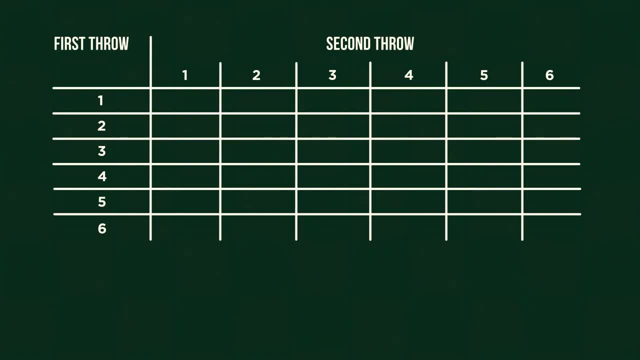 Firstly, we should draw the required sample space. We can then highlight the outcomes which match the question. There are nine crossover points, so nine outcomes that work for us. Because there are thirty-six possible outcomes? our answer is nine over thirty-six, simplified to one quarter. 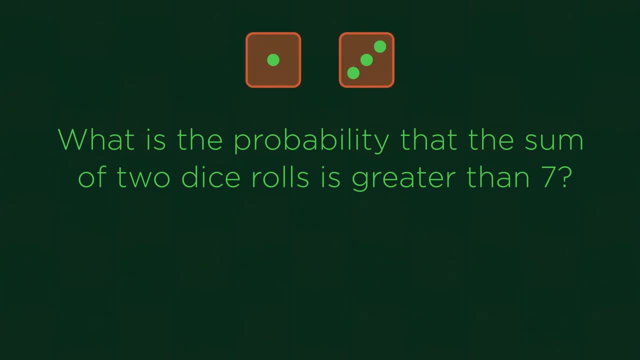 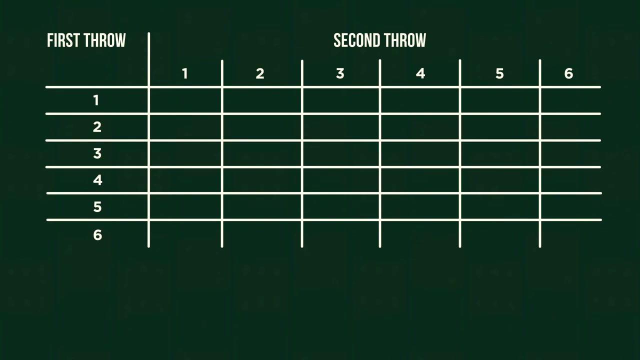 Now have a go at this different example. What's the probability that the sum of two dice rolls is greater than seven? Pause the video and resume when ready Again. we can use this sample space, this time to list the sum of outcomes of the two events. 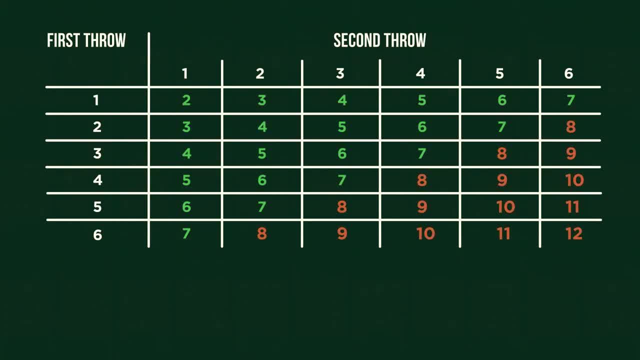 When we add in the sum values and highlight the answers larger than or equal to the sum of outcomes. Again, we can use this sample space this time to list the sum of outcomes of the two events. When we highlight the answers larger than or equal to the sum of outcomes. 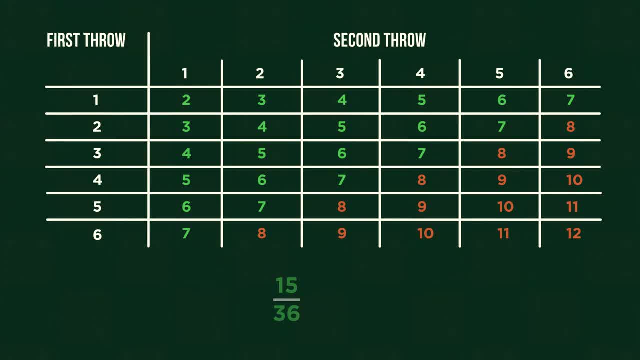 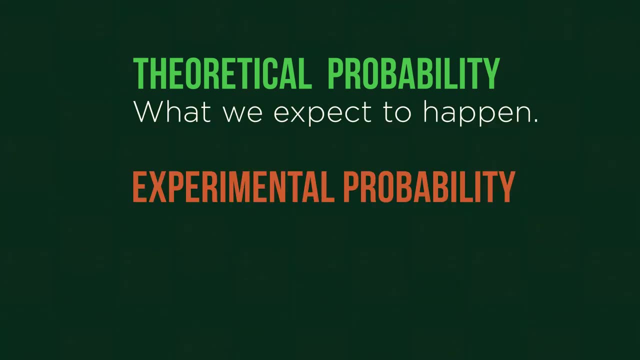 we can see that there are fifteen outcomes that work. Fifteen out of thirty-six potential outcomes leaves us with the probability five over twelve. when simplified, These outcomes are, of course, entirely theoretical. Theoretical probability is what we expect to happen, whereas experimental probability is what actually happens when we test the situation. 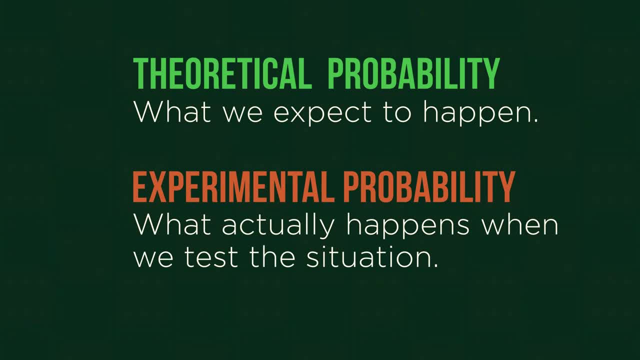 Generally, the more we try, the closer the experimental probability gets to the value of the theoretical probability. Generally, the more we try, the closer the experimental probability gets to the value of the theoretical probability. Generally, the more we try, the closer the experimental probability gets to the value of the theoretical probability.